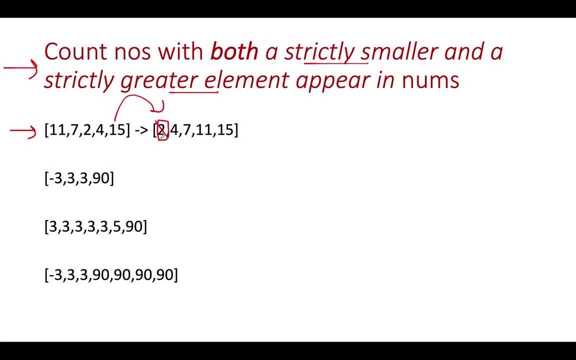 element than it in the array No. So this will not be part of the answer. Let's proceed ahead. Next we have is 4.. 4 has a strictly smaller element. 4 also has a strictly greater element. So any of these elements- 7,, 11 and 15- contend for a strictly greater element than 4.. 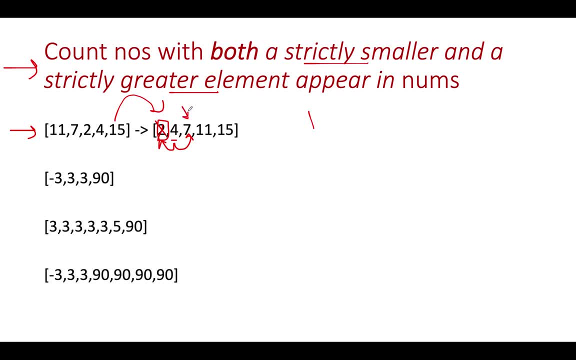 That means we have identified one such number. Let's proceed ahead. Next we see 7.. 7 has a strictly smaller element. It could be either 4 or 2.. Also, it has a strictly greater element. It could be 11 or 15.. The count gets updated to 2.. Let's proceed ahead. Next we have 11.. For 11, we have: 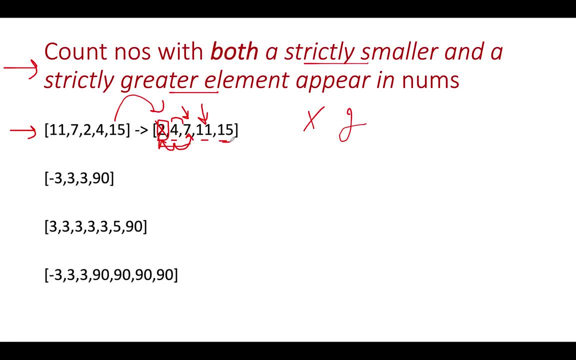 3 possibilities of strictly smaller elements and 1 possibility for a strictly greater element. The counts get updated to 3.. Let's proceed ahead. Next we see is 15.. For 15, we have 4 possibilities for smaller element. There is no possibility for greater element, And the answer finally turns out. 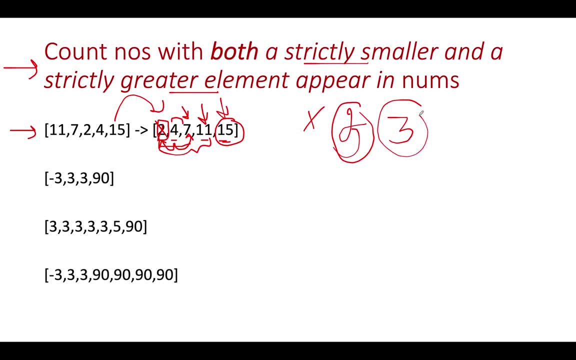 to be 3.. What is the key point? The key point is that we understood from this example. We understood that the minimum element and the maximum element will not contribute to the answer, because for the minimum element, there will be no element which is smaller than that and for the maximum element, there will be no element. 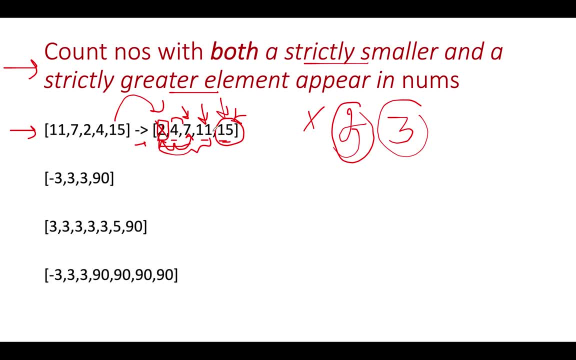 in the array that would be greater than that, As a result of which min and max will never contribute to the array. Let's proceed ahead and let's walk through another example. Here we have specified as minus 3, 3, 3 and 19.. Let's proceed ahead and let's walk through another example. Here we have: 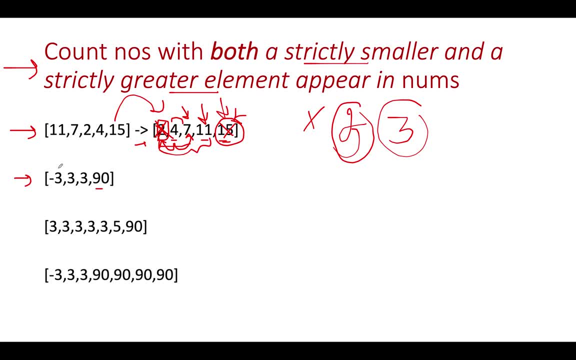 3.. It's actually sorted in nature by coincidence. So we understood that the minimum one will not contribute to the array. The maximum one will not also contribute to the array. What is left? It is left with only two elements, which is 3, 3, and the answer becomes to be 2 in nature. So the answer is: 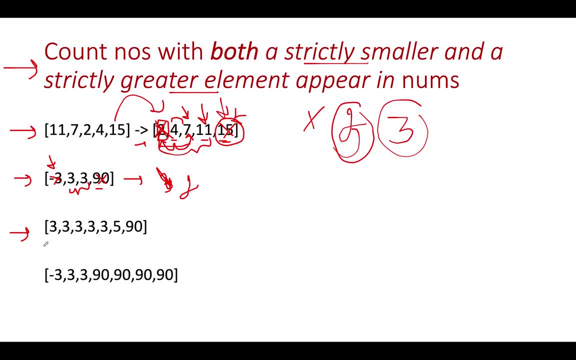 2. Let's proceed ahead. This is an interesting case. We have an array as 3, 3, 3, 3, 3, 5, 90. And, as you can see, the minimum element occurs multiple times. 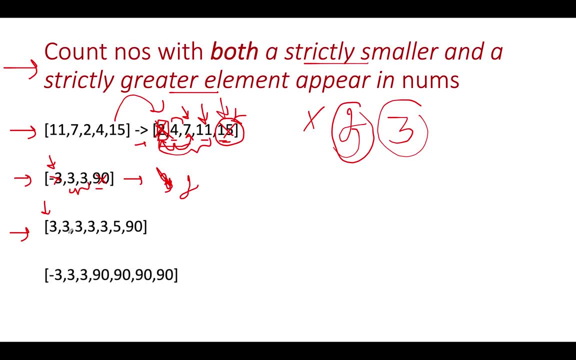 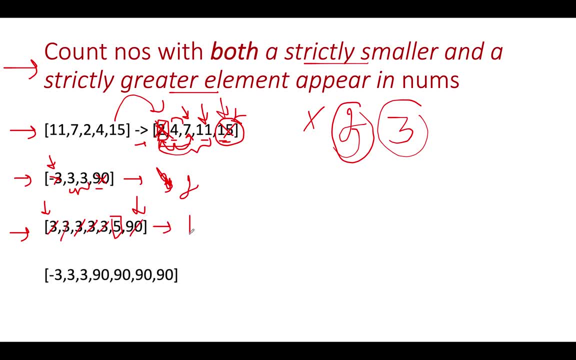 element, which also gets skipped, So the answer becomes 1.. Similarly, here in this case we can see multiple entries for the maximum element, So all such instances get skipped, and what is left Is these two elements: 3, 3.. There is a minimum element minus 1, which also gets skipped, So the 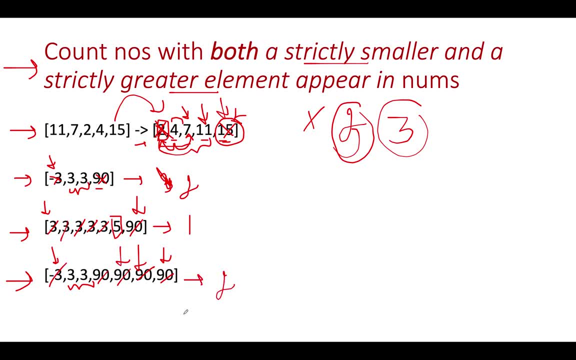 answer becomes 2.. I hope you understood this logic, these various test cases, and now let's talk about how can we go about it. The first and the foremost approach is pretty simple and straightforward: What you can do: You can find out the minimum element and you can find out the 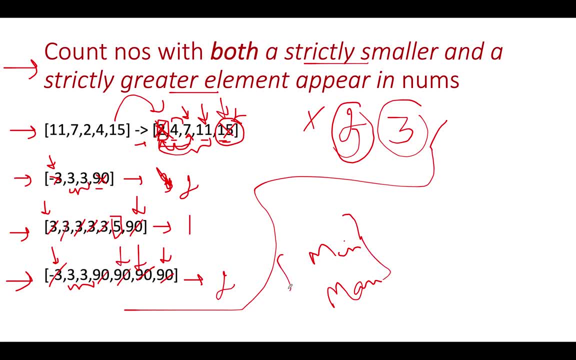 maximum element in this input array. Store them in two variables. Then you start the iteration If your current element lies within the range of this particular two elements, in that case you increment your count variable. Otherwise you simply skip it whenever the current element happens to be either equal to the minimum one or the maximum one. In the end, 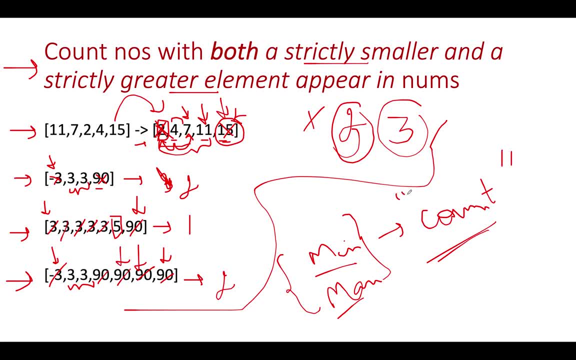 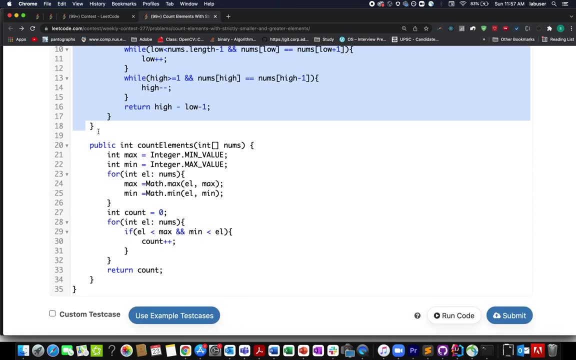 whatever count variable is held, you simply return it out. Now let's quickly jump on to the coding section, where we'll conclude the approach. So let's get started. I'll walk you through the two solutions that I have provided. The one that I just talked is this one: 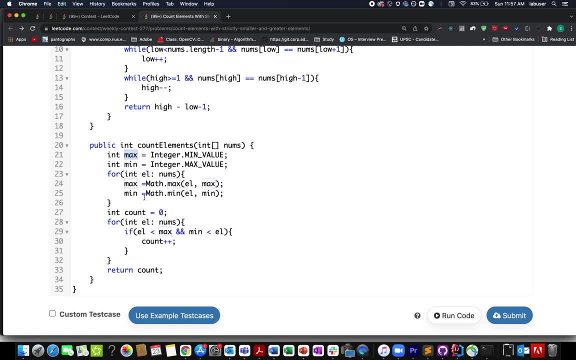 You go and find out the minimum element and the maximum element from this input array. You create a count variable. If your current element happens to be within the range of max and min, you increment that count and return that value in the end. The other possible way is to sort this array up You. 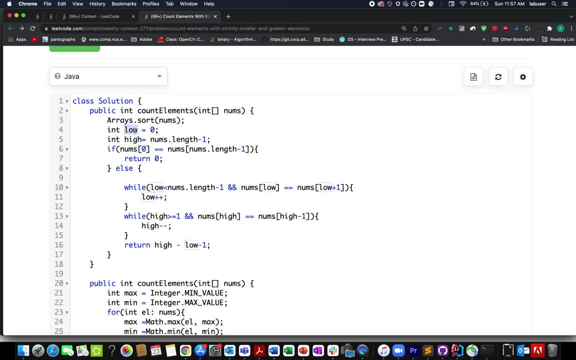 create a low pointer. I'm using the two pointer approach here: Low pointer and high pointer. If my current element the lowest element in my array, after sorting it out, it will be equal to the highest element in my array, the last element, Then in that case we simply return zero because 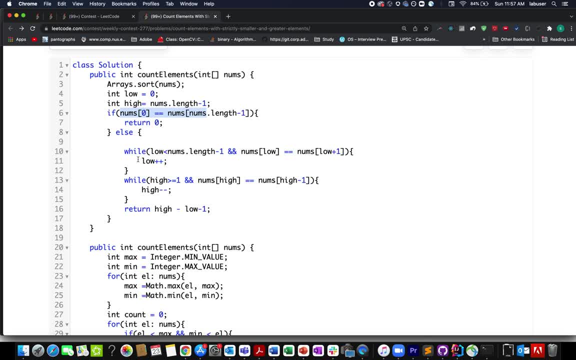 all the elements tend to be equal in nature. Otherwise, I keep on incrementing till the time I'm seeing the low pointer as the minimum value. So in case my low happens to be equal to low plus one, I simply increment my low pointer. Similarly, I keep on decrementing my high pointer till the